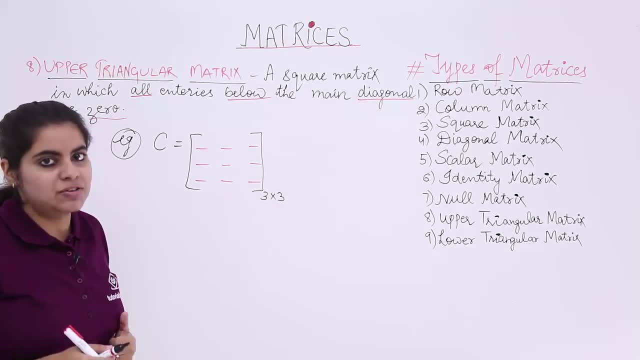 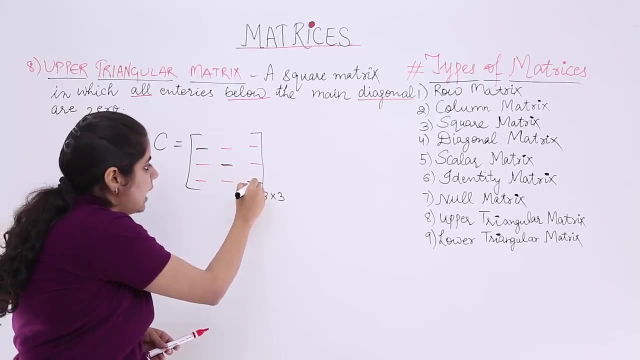 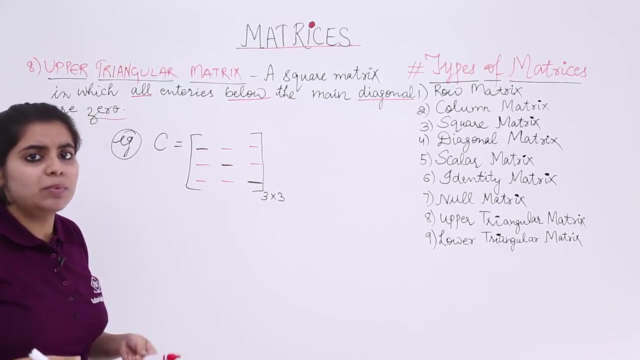 of elements for a 3 ordered square matrix. Now, what will be the diagonal entries? The diagonal entries will be which are blackened. These will be the diagonal entries and these diagonal entries are basically a11, a22, a33.. Now suppose these diagonal entries are something. 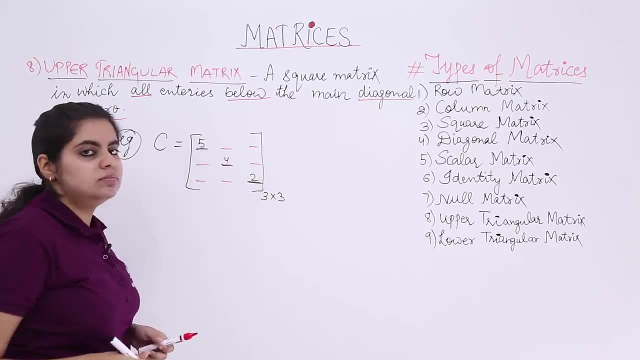 as 5,, 4, 2.. So what will be the diagonal entries? So these are the diagonal entries that are blackened And the elements above the diagonal. if this is the diagonal comprising of 5,4,2, the elements. 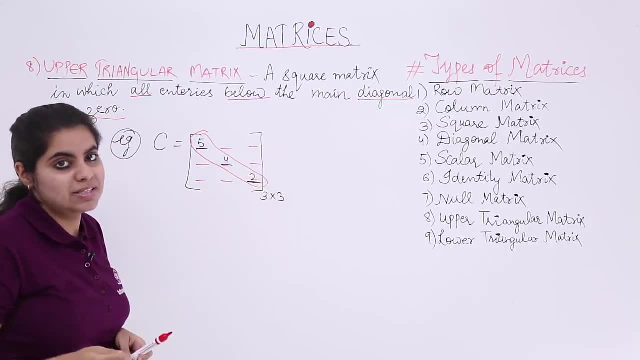 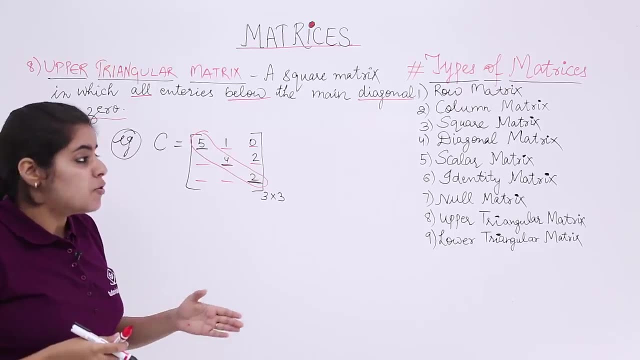 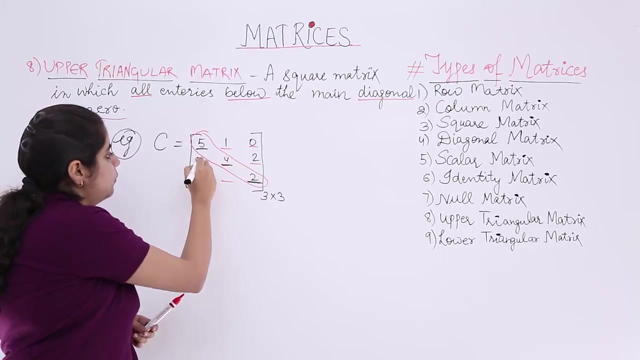 above the diagonal are this region, 3 elements and they are supposedly something 1,0,2.. So my upper triangular matrix would be 1. where in all the elements, where in the diagonal is there, all the elements below this diagonal are 0.. 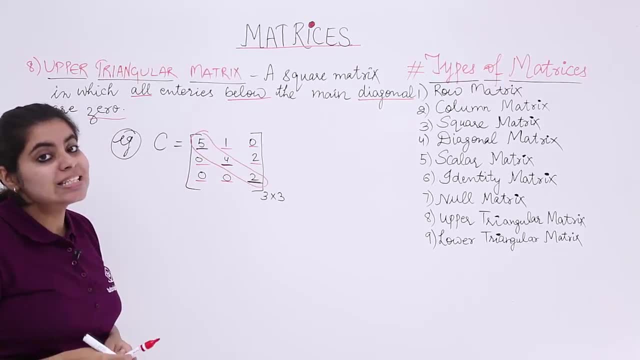 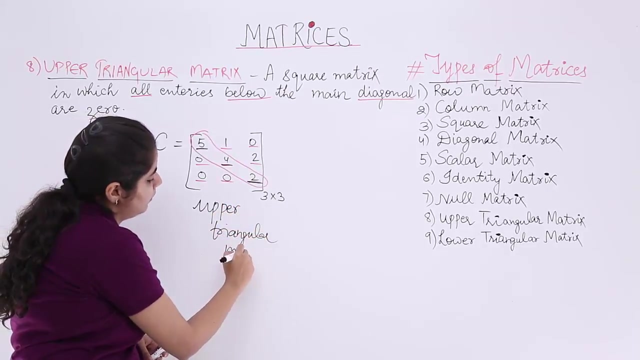 You see, the elements below the diagonal are 0. so yes, it is upper triangular matrix. The elements above should not be 0. One can be 0, all should not be 0, right? So it is upper triangular matrix. and again I will be showing with the help of another. 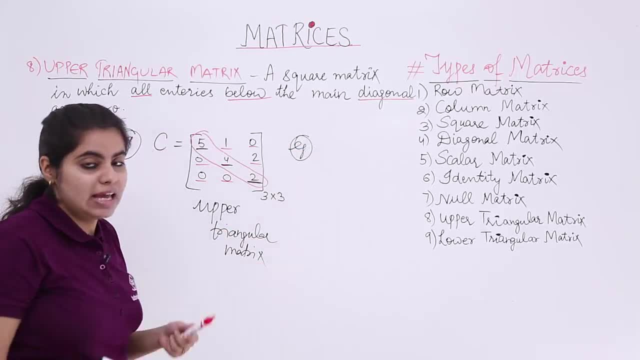 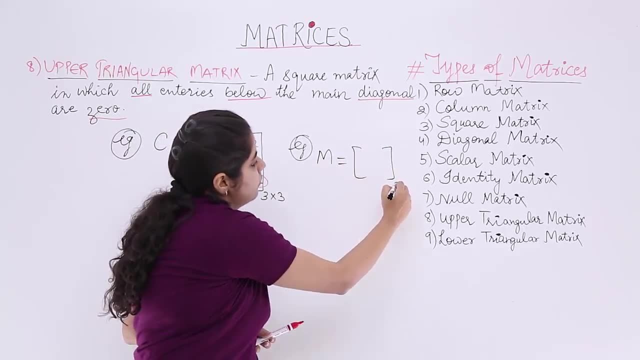 example, for those people who find it a bit confusing, I have again a matrix, say it is M And this is the upper triangular matrix. This M matrix is a 2x2 matrix. it cannot be a 2x3 or 3x4 matrix because it has to be a. 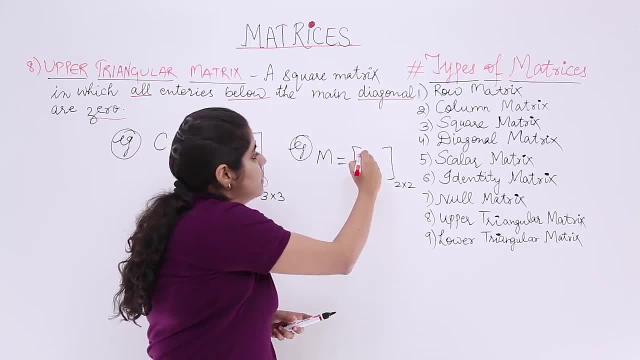 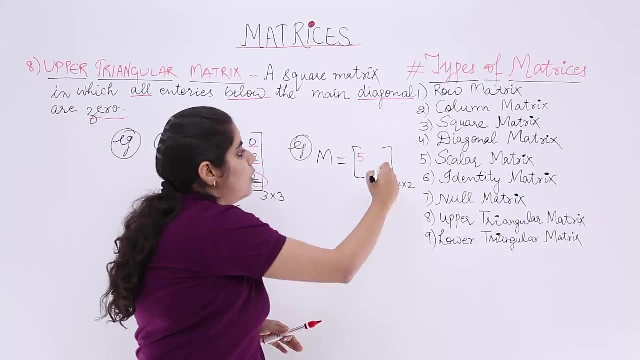 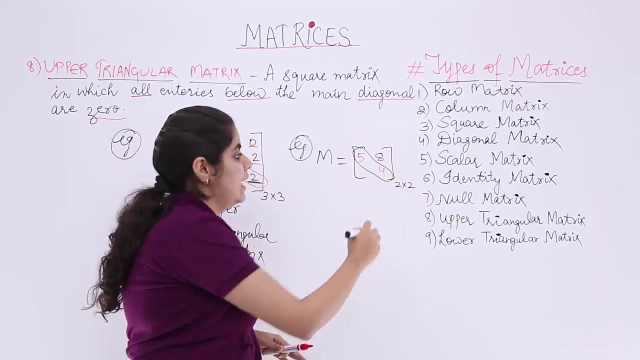 square matrix, A 2x2 matrix, and the elements are given to me as 5 and 4. these elements are for the diagonal. The element above the diagonal is what. the element above the diagonal is given to me as 8.. This is the diagonal element above the diagonal is 8. below the diagonal is 0, since the element 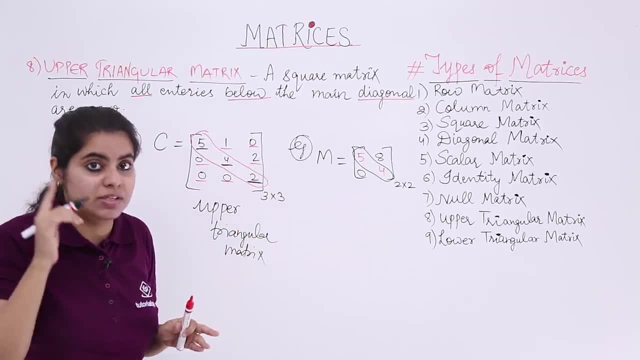 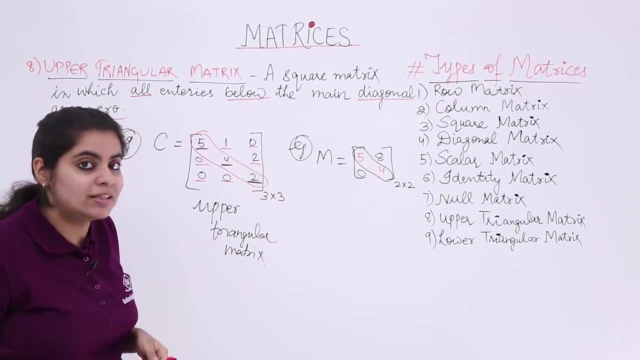 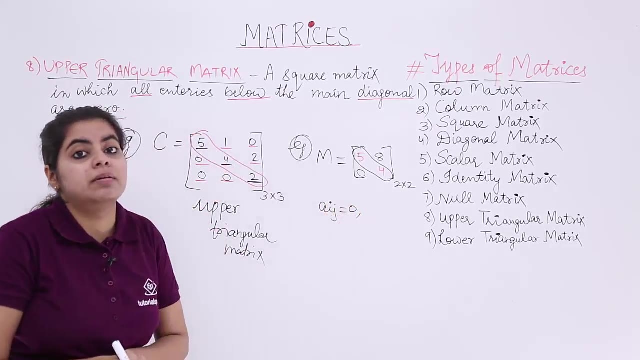 below The leading diagonal or the main diagonal in a square matrix is 0. it is what it is: upper triangular matrix. And now you have understood. let's now write it in the form of a mathematical formulation that here we have: aij is equal to 0 when aij is equal to 0 for the elements below the diagonal.